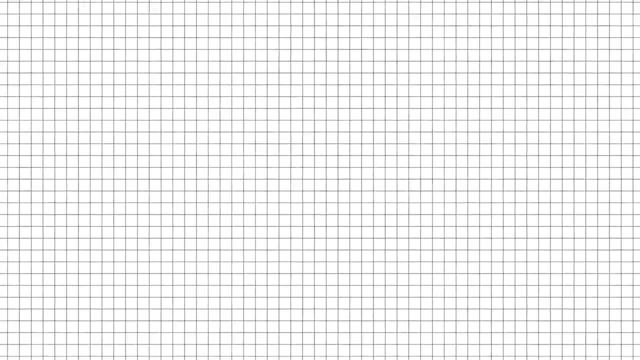 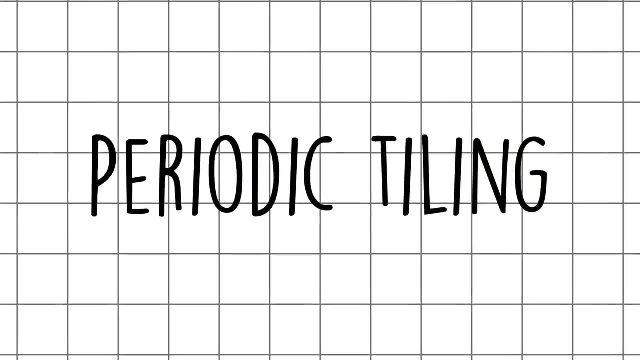 Theoretically, you can extend this pattern out to infinity in all directions. Think of it like tiling an infinitely big bathroom floor. A periodic tiling is when you can copy the entire pattern, slide it across and lay it perfectly onto itself. 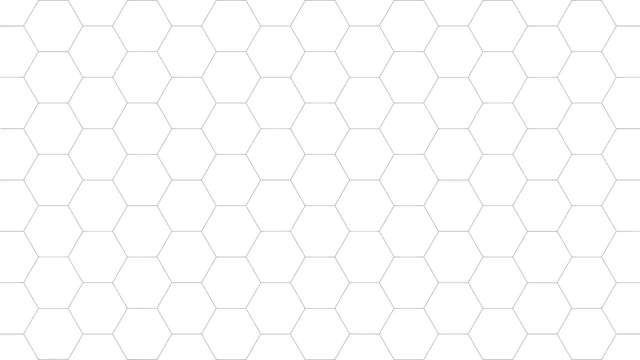 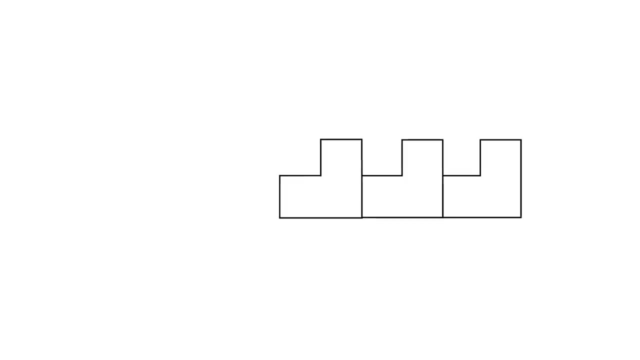 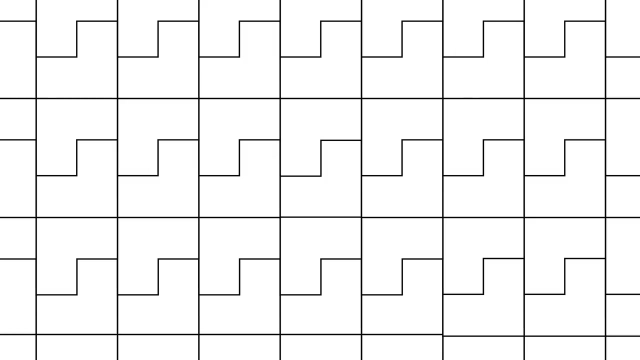 This is called translational symmetry. Periodic tilings are common and can be made of more than one shape. Some shapes that make up periodic tilings can also be arranged in ways that do not have translational symmetry. When we arrange this L-shaped tile like this, it makes a periodic tiling. 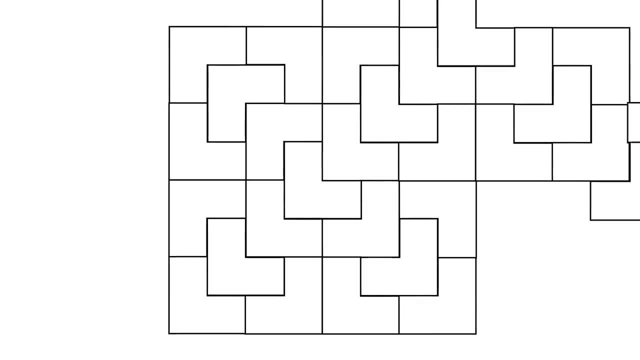 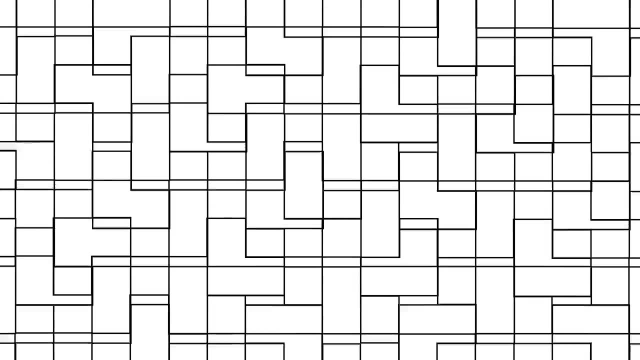 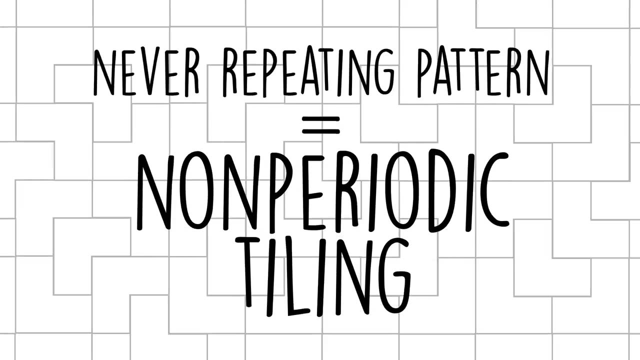 But if we arrange it like this, no matter how we slide it around, we can't get it to overlap with itself. Tilings like this are called non-periodic, and when we say never-repeating pattern, this is what we mean. 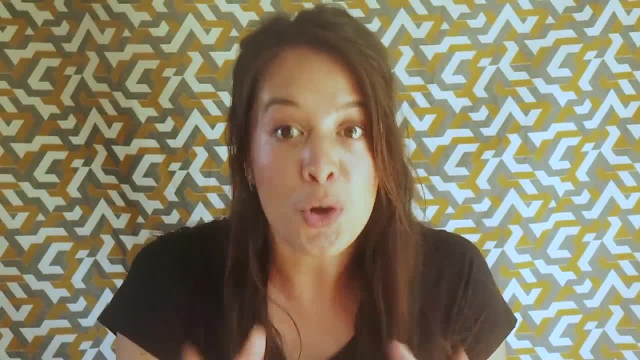 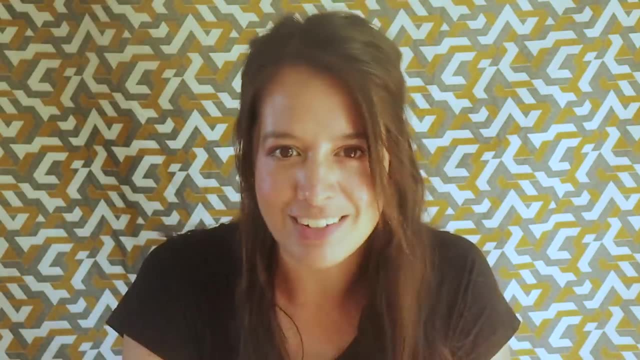 This got mathematicians thinking: Are there shapes that can only be tiled non-periodically, That, no matter how you arrange them, it's impossible to create a repeating pattern? Such tiles are called aperiodic tiles, and for a long time no one knew if they existed. 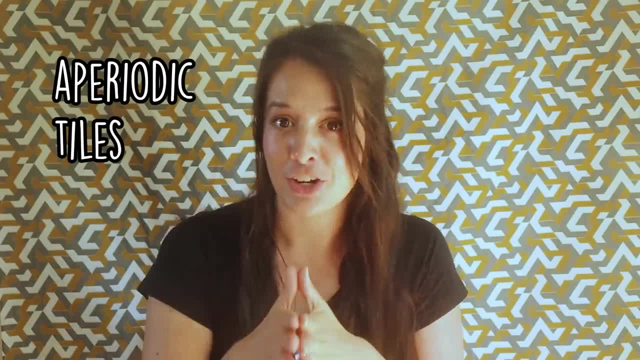 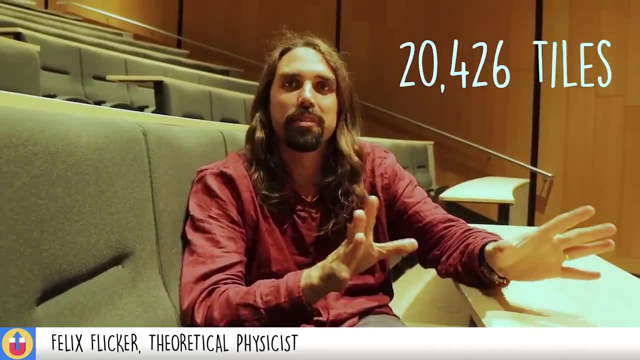 Then, in 1964, the first set of aperiodic tiles was discovered, The original set of tiles that had this property. there were 20,426 of them, So different tiles, And then rapidly that set got cut down and down until someone found a set of six tiles that could do it. 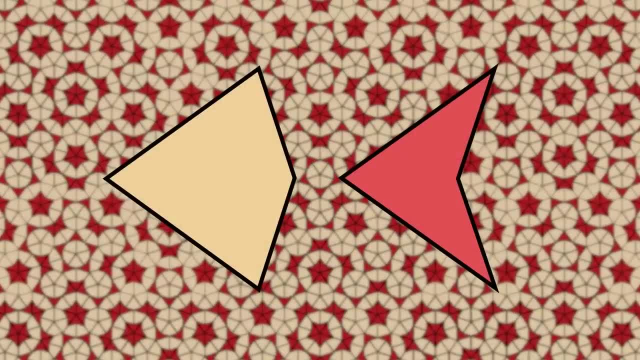 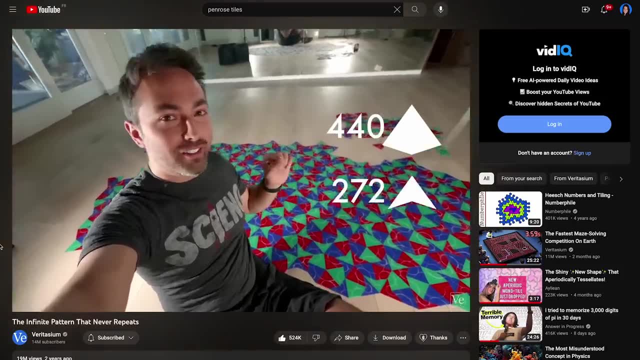 And then Roger Penrose's work brought it down to two tiles And then I think it was uncertain as to whether it could go down to one. Veritasium has an excellent video about Penrose tiles. I've linked it in the description. 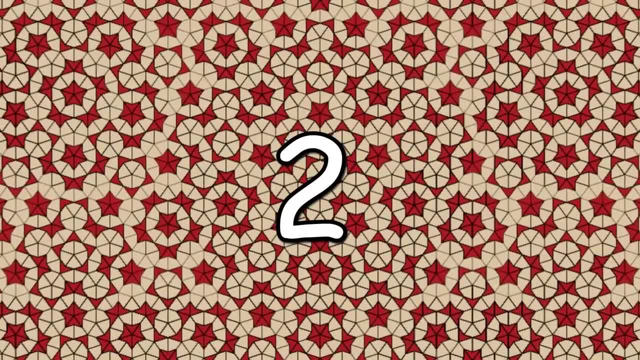 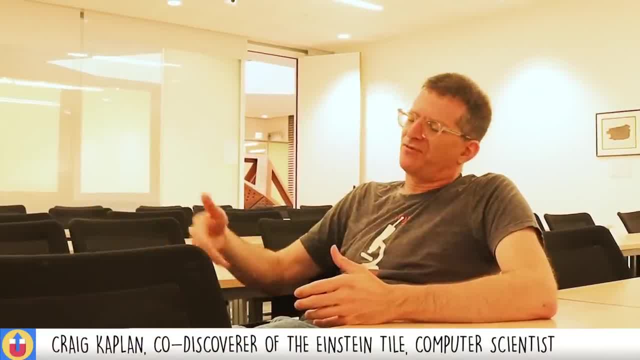 Since the 60s, Penrose tiles have held the record for the smallest number of aperiodic tiles. And then we hit the wall right. It was obvious that the last step we wanted was to find a single shape that could only tile aperiodically. 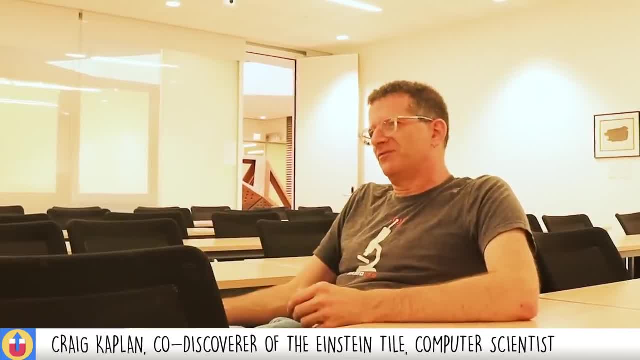 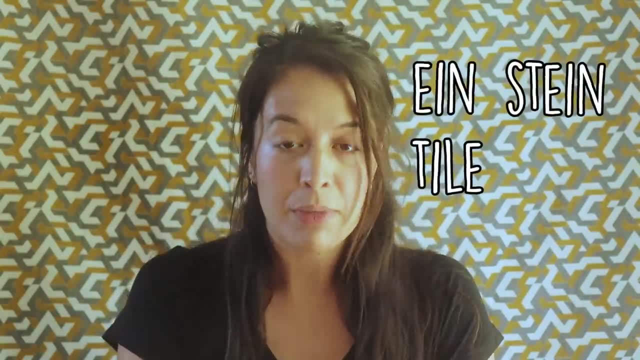 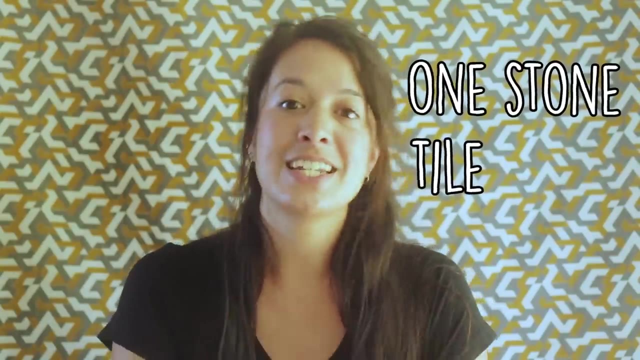 And for roughly 50 years nobody was able to find one, And so the race for the single aperiodic monotile was on. It was called the Einstein tile, meaning one stone in German, And now, in March of this year, it was discovered by a retired printing technician. 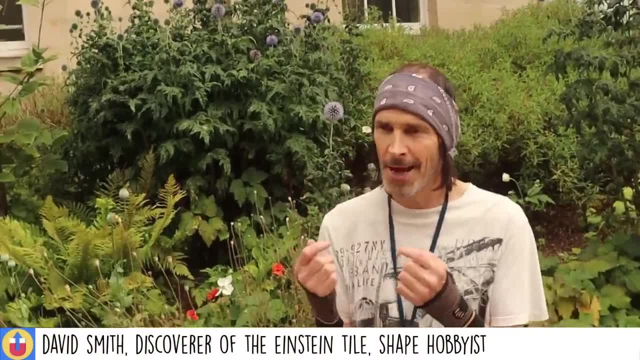 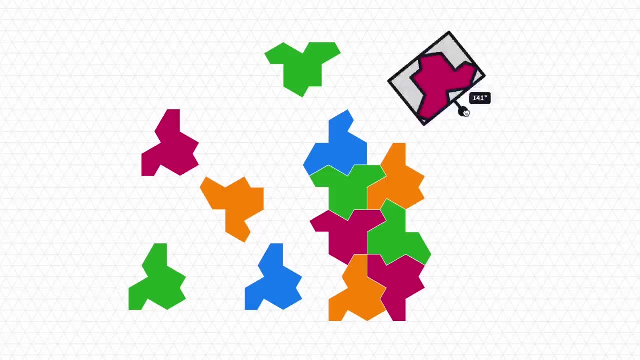 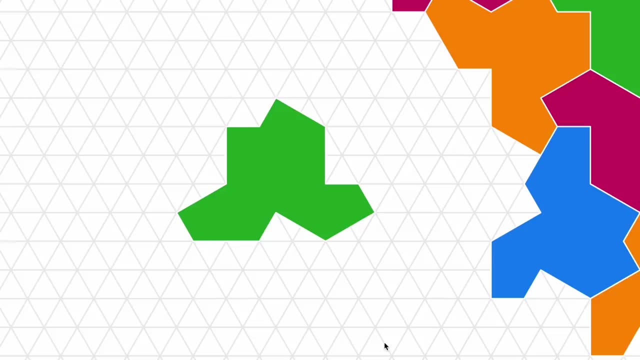 David Smith, who describes himself as a shape hobbyist. I'm just a bloke off the street, You know, just playing with shapes. David was playing around with shapes on his computer when he discovered a very simple shape that behaved strangely. It's called a polykite because it's made up of eight kite shapes. 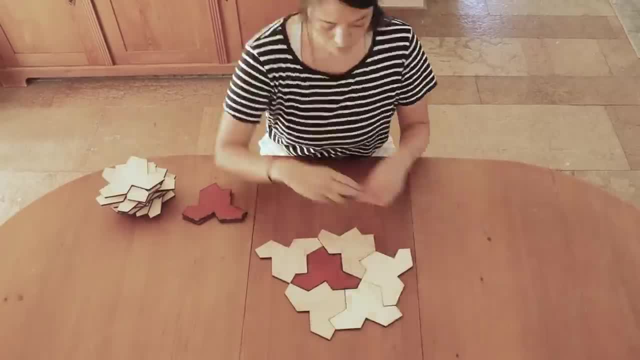 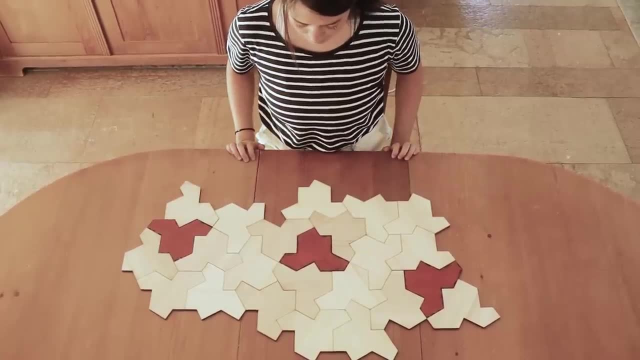 You can get it just by cutting up hexagons. He printed out copies and began to tile them by hand. The funny thing was he couldn't get them to tile periodically. I've never seen them. That's weird, you know. 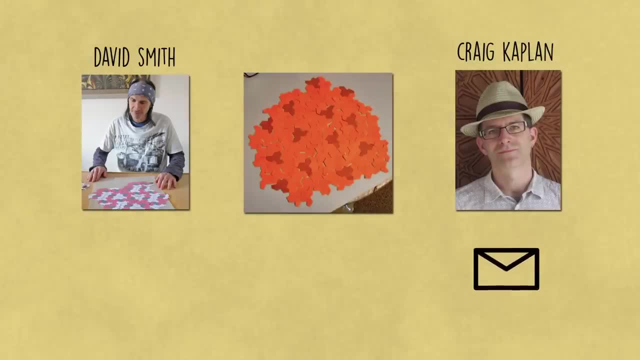 He felt he was onto something. So on November 20th 2022, he emailed Craig Kaplan, a computer scientist from the University of Waterloo. Could this be an answer to the Einstein problem? Now, wouldn't that be a thing? 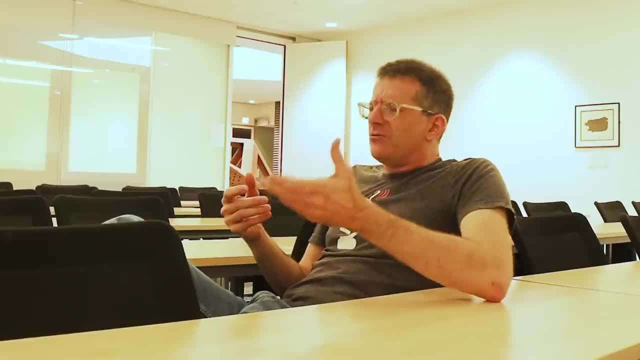 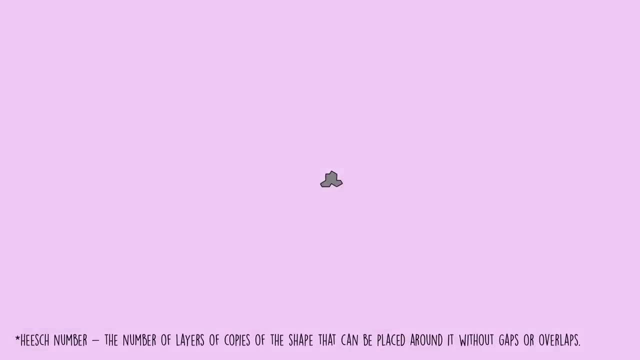 We now know that it was indeed a thing He had reached out to me because of this previous work I had done that can use computer software to compute H-numbers So it can try to surround and surround and surround and see how far you can go. 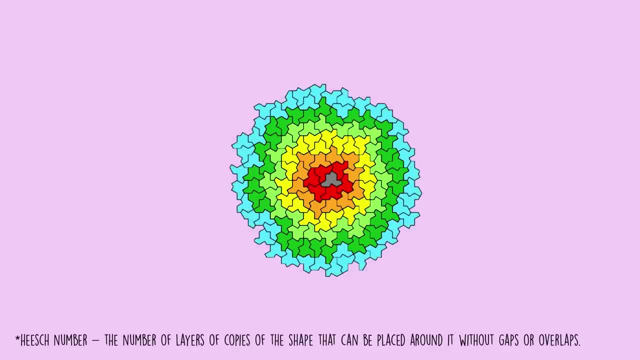 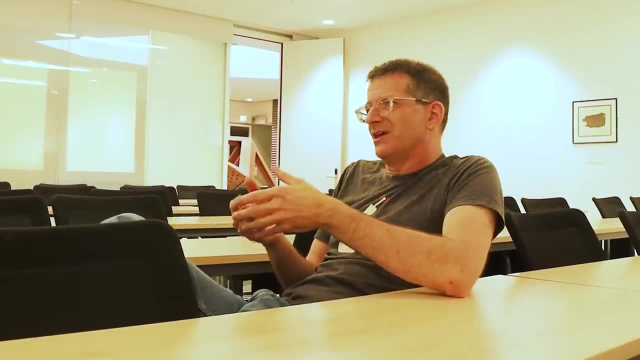 And my software said: you can go as far as you want. As far as we could tell, you never run out of the ability to grow a patch of tiles. That means there's some faint possibility that this is it, that this is the aperiodic monotile people have been looking for. 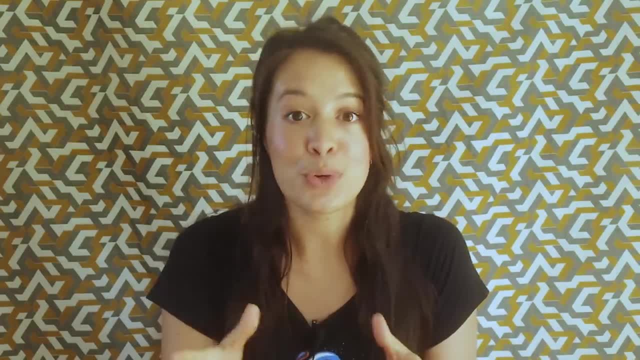 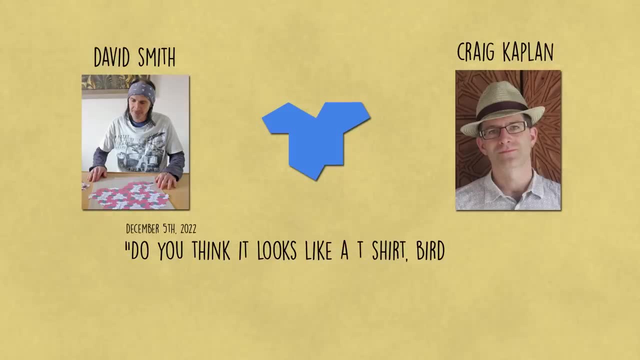 While they were investigating its potential as the Einstein tile, there was also the task of giving it a name. On the 5th of December, Dave emailed Craig: do you think it looks like a t-shirt? bird in flight, some sort of boot? 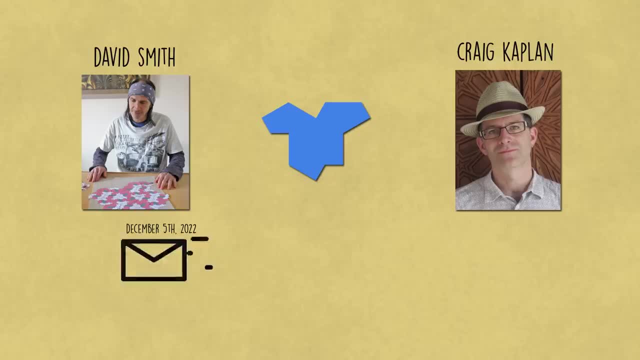 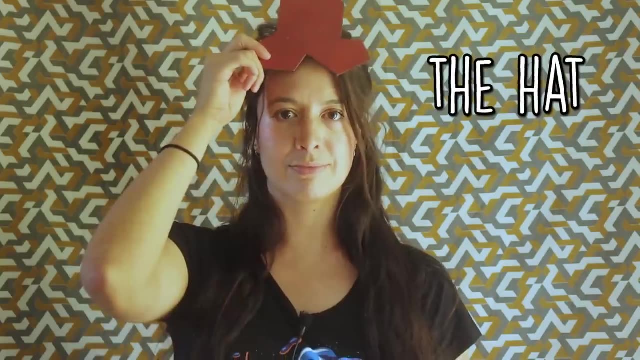 weird fish or something else. Craig replied. family members think it looks like a shirt, Maybe a hat, if you turn it upside down, And so it was named the hat. Now the money question. How do we know that the pattern never repeats? 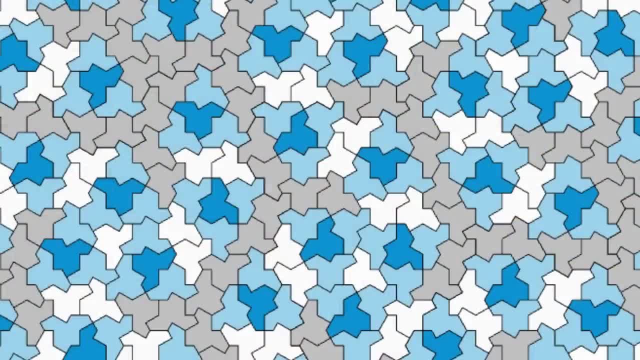 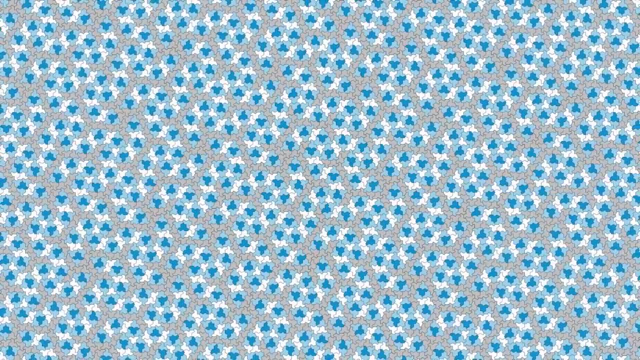 Sure, it doesn't look like it repeats when you look at a segment, but we're dealing with an infinite plane. Maybe there is some ginormous translation where the original tiling and its copy line up. To be sure, we need a mathematical proof. 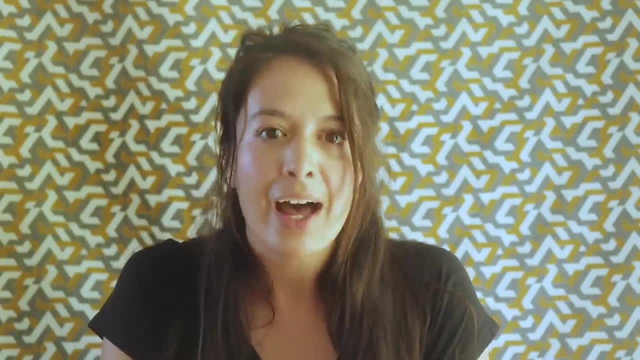 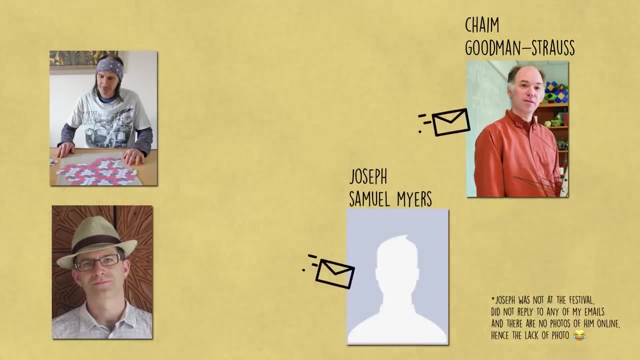 It was here that Dave and Craig called in reinforcements: Haim Goodman Strauss, an American mathematician working in geometry, and Joseph Samuel Myers, a software engineer working in combinatorics. They immediately jumped on board. I mean, of course it's a big deal to me. 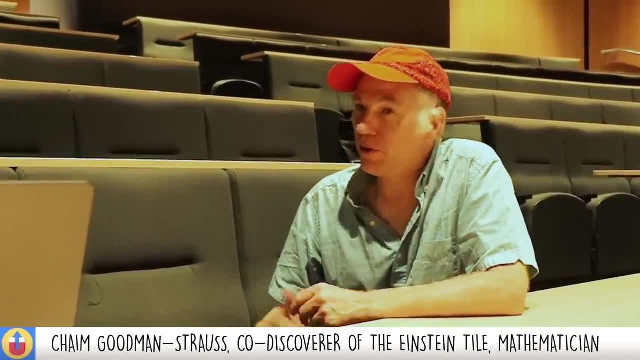 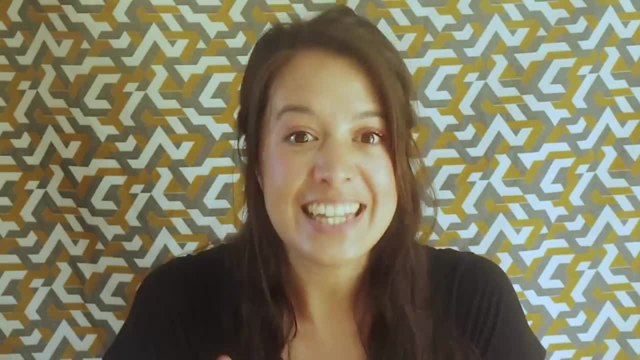 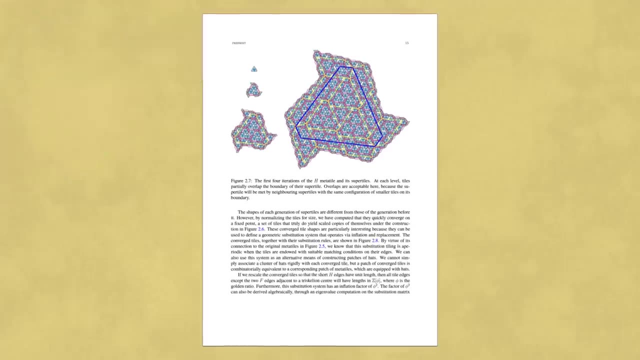 It answers a long-standing question that everybody that is involved in this has wondered about. Just eight days after joining forces, the team derived a mathematical proof sealing the hat's identity as the long-sought-after Einstein tile. Diving into a foolproof would involve some heavy mathematics and computer science, so I'm going to. 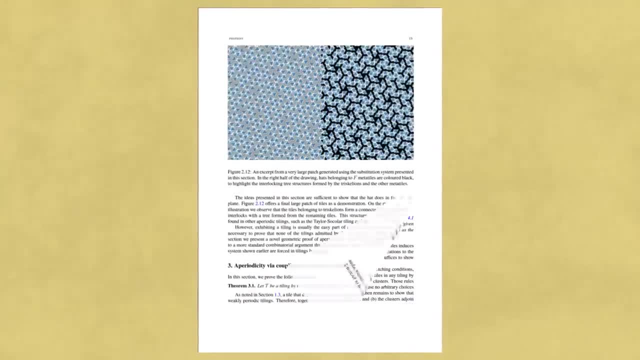 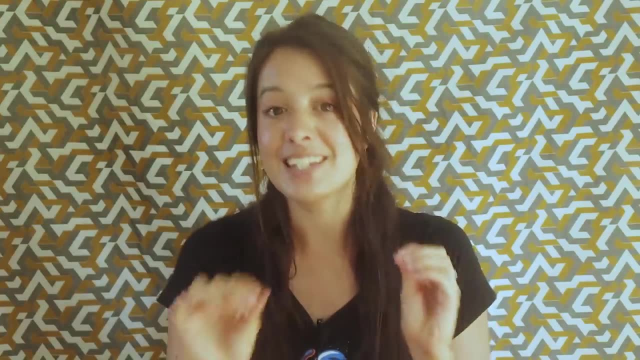 go into all the details here, But I really want you to get a feel for the genius behind proving the hat's aperiodicity, so what I'll do instead is give you an overview of the main technique that was used and show how the team applied it to the hat tiling. 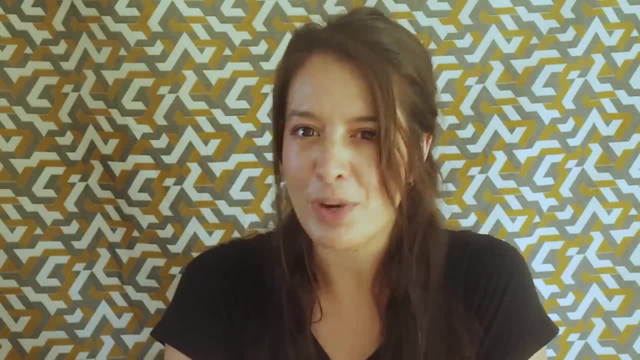 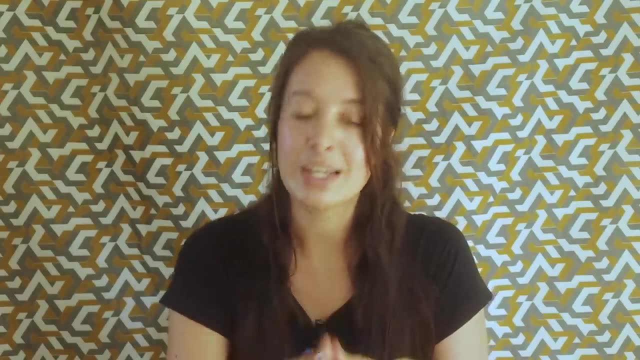 By the way, this is far from the end of the story. There are more surprises to come, Infinitely more, actually. Okay, so at the core of the proof is a classic technique in tiling called the unique hierarchy method. In a nutshell, this method is called the unique hierarchy method. 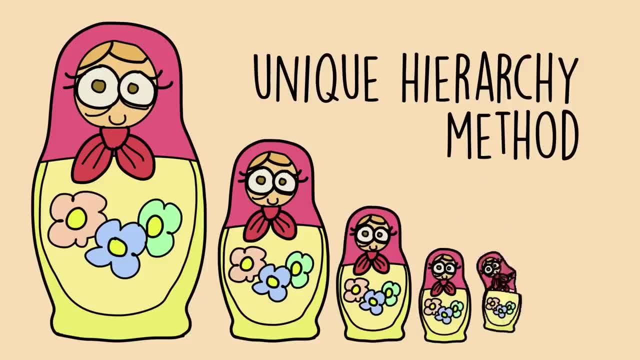 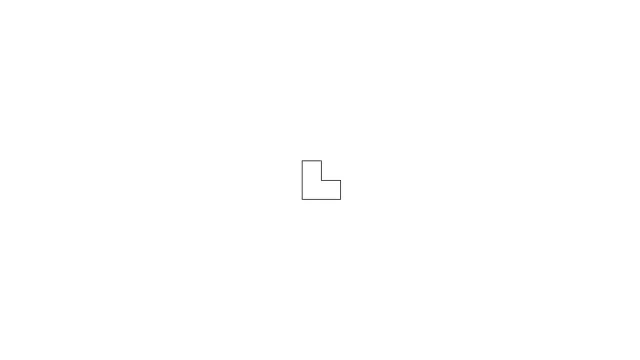 In a nutshell, this method is called the unique hierarchy method. This method is called the unique hierarchy method. This method relies on the hierarchical or fractal nature of a tiling. Take this non-periodic L-tiling from before. It starts with a single L-tile, then makes copies of itself to form a larger L. 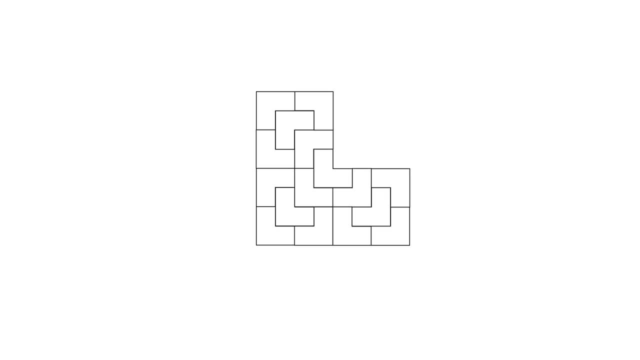 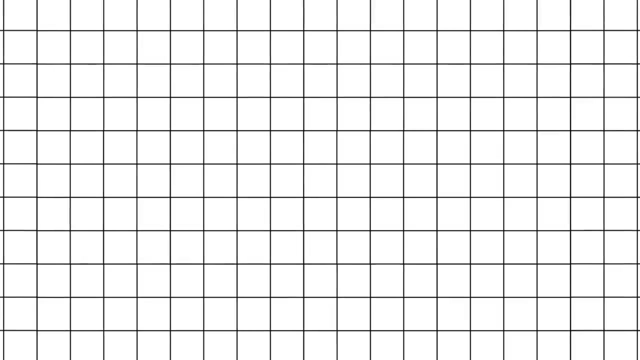 then makes copies of that larger L to form an even larger L, and so on until it covers the infinite plane. This periodic square tiling is built in the same way: Start with a single square tile and copy it to make larger squares, But there's a big difference between the L-tiling and the square tiling. 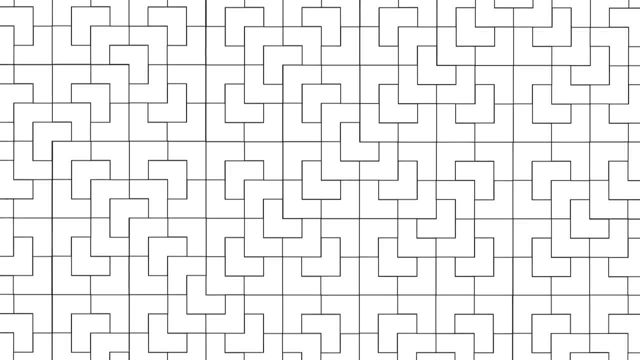 Any L, no matter its size, belongs to only one L of the next size up. This L belongs to only this one bigger L, And that L belongs to only this one bigger L, And that L belongs to only this one bigger L. 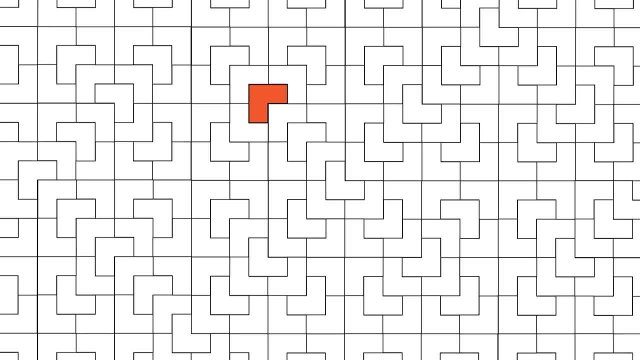 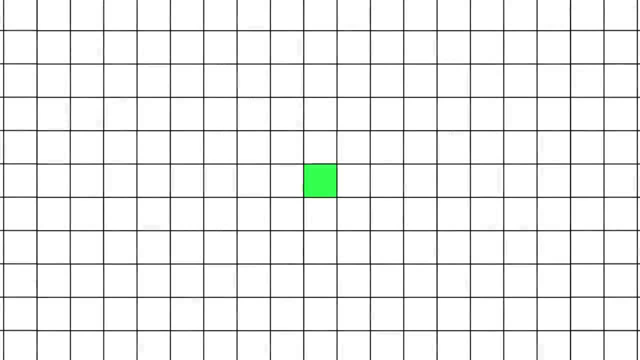 Try it for yourself. Starting with this L-tile, can you figure out which bigger L-tile it belongs to and which one that belongs to? Now try it with the squares. It doesn't work. This square could belong to any one of these bigger squares. 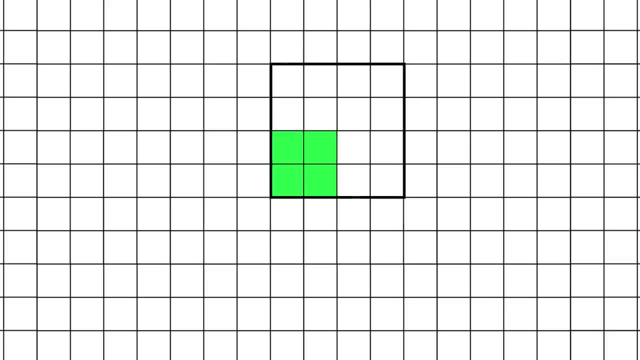 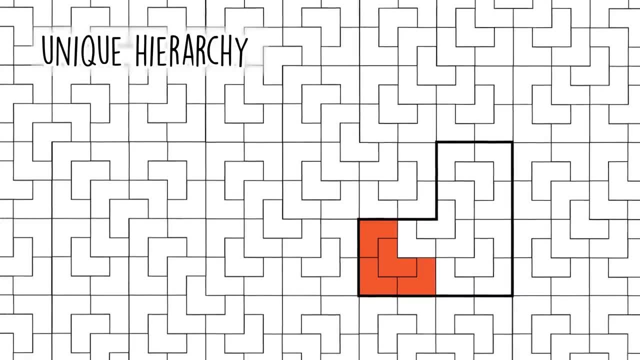 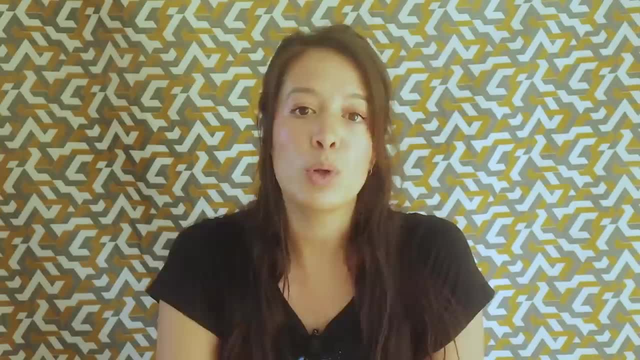 And that square could belong to any one of these bigger squares. This is the essence of unique hierarchy: Each smaller tile belongs to one and only one unique larger tile, And that guarantees non-periodicity. How Well, one way to think of a periodic tiling is that. 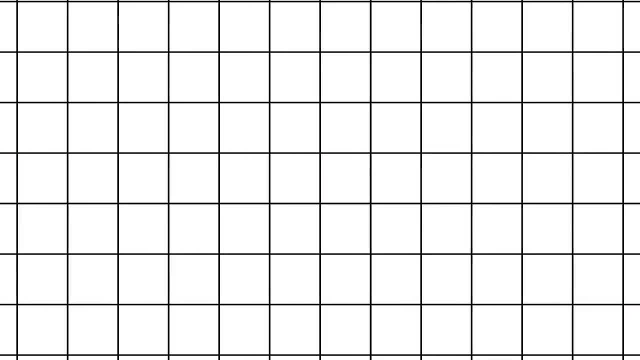 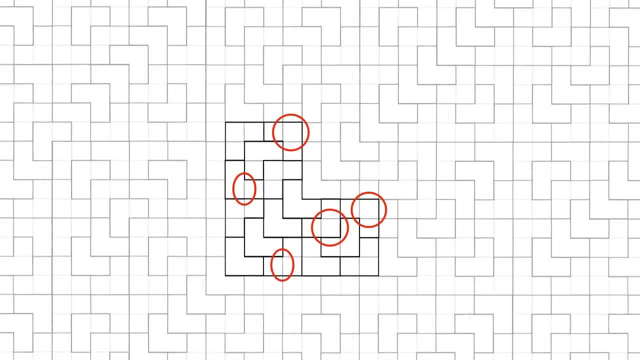 you can copy and translate it on top of itself And it looks unchanged. So now imagine copying a segment of our L-tiling and shifting it on top of itself. Right off the bat we can see it doesn't align perfectly, But even without visual cues we can prove that it's different to the original. 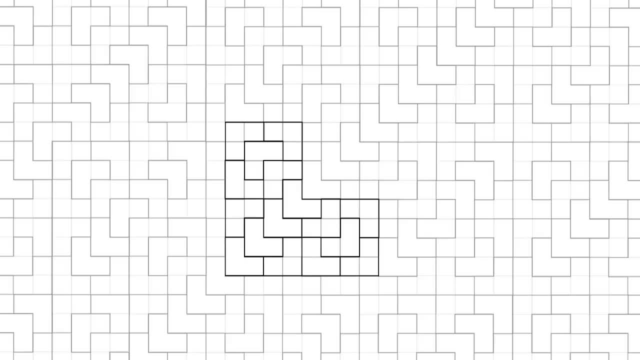 As we know, in the original each L belongs to only one larger L, But in our shifted version, this tile belongs to two larger Ls. You might think, okay, well, what if we just copy and translate it on top of itself? 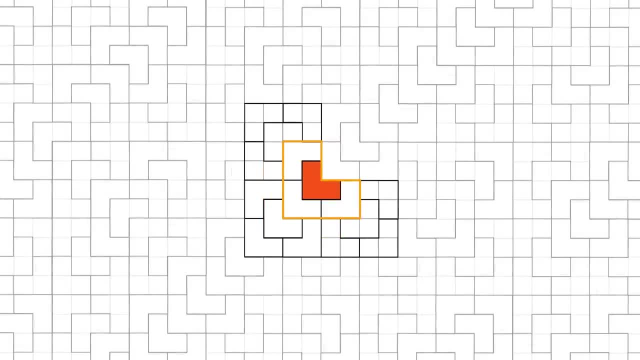 We could just make the translation bigger so that it doesn't belong to both Ls anymore. But that doesn't fix the problem, Because this larger L belongs to these two larger Ls Because of the uniquely hierarchical nature of the tiling. 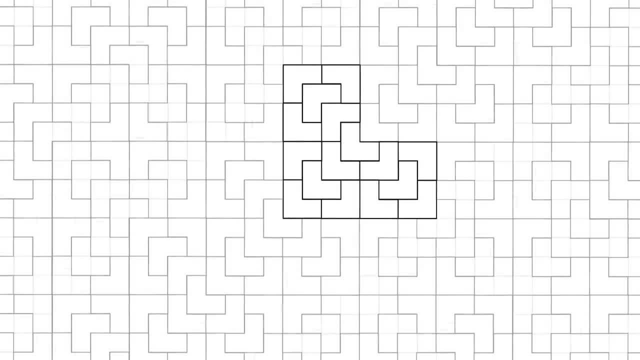 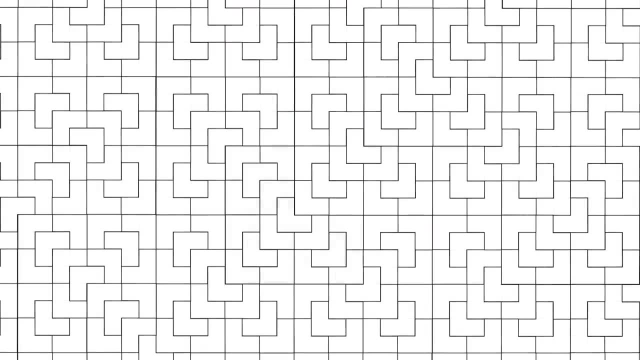 no matter how big of a translation you make, there will always be a larger L that belongs to two even larger Ls. This means that it will never be the same as the original tiling, where every L belongs to only one bigger L. 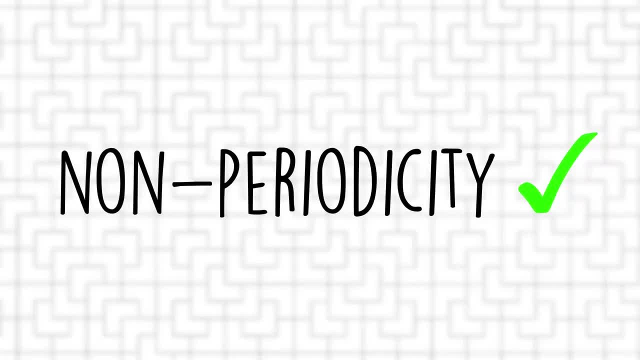 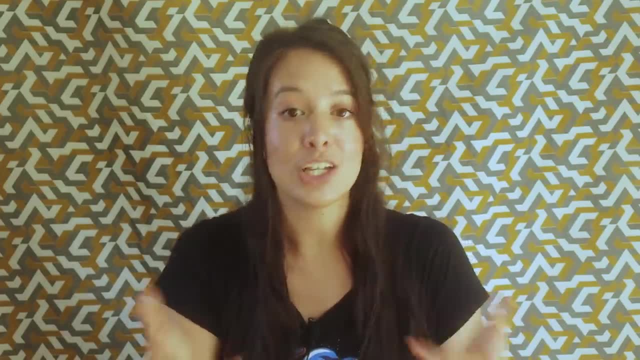 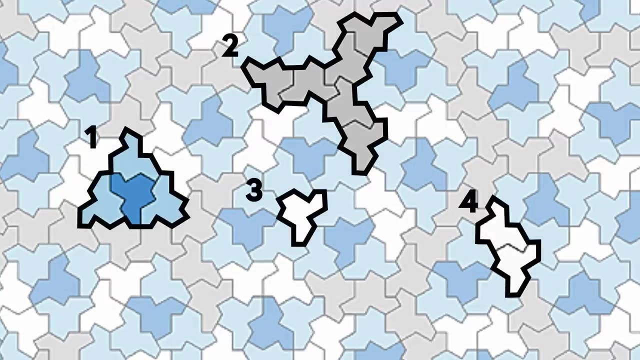 That is how we guarantee non-periodicity. The researchers used this idea to prove that the hat tiling is aperiodic by showing that it must be built in a unique hierarchy. They started by identifying four reoccurring clusters of hats. They realised that the entire plane could be tiled with just these four clusters. 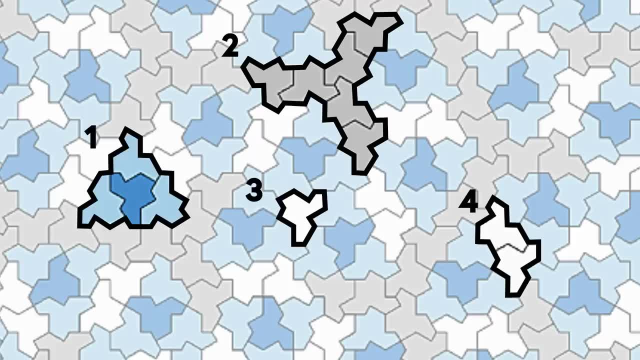 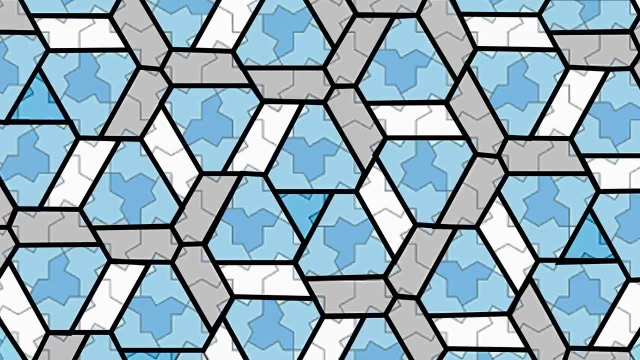 To make things easier to work with, they replaced the clusters with what they called metatiles. Now the entire plane could be covered with these four clusters. They began to focus on just the metatiles and put the hats out of their mind for the moment. 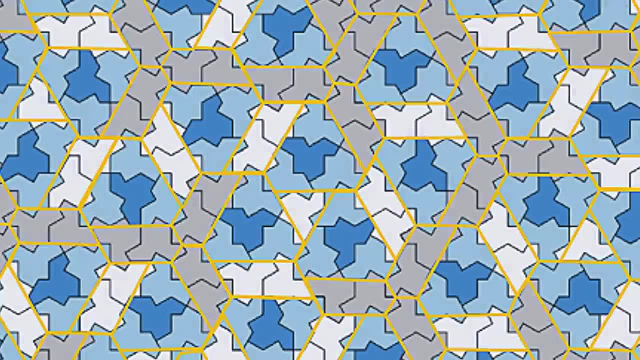 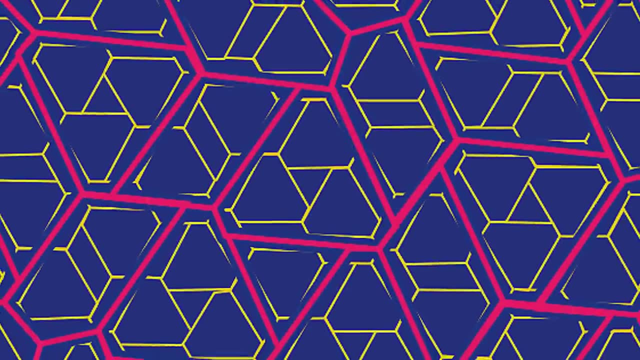 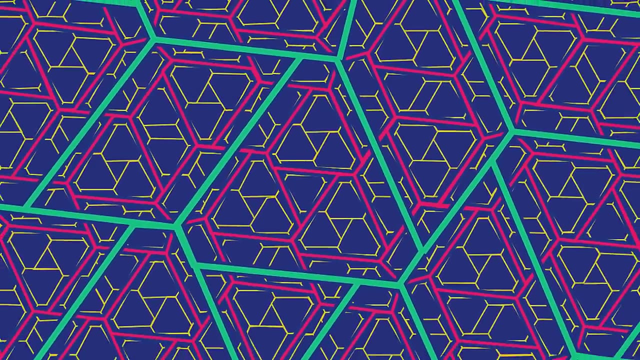 They could always bring them back at any time. They showed how these metatiles formed larger and larger versions of themselves And, just like the L-tiles, the hierarchy was unique. Basically, the hierarchy is a set of four metatiles. 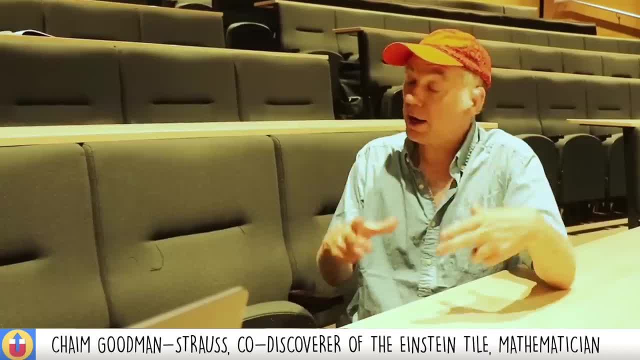 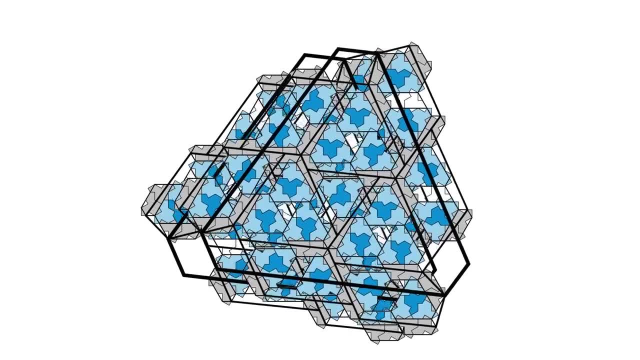 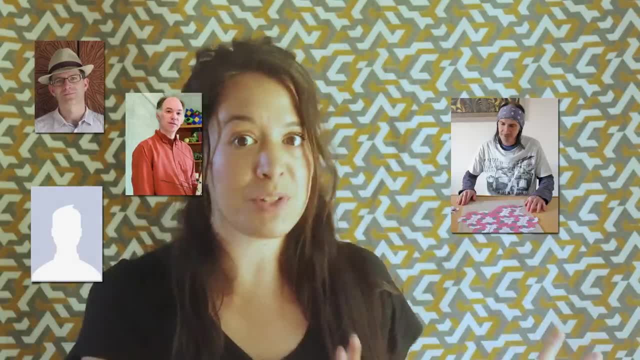 You have these larger and larger structures, and any translation would be smaller than one of these structures within the tiling. While these guys were busy hashing out the proof, Dave was busy too. He'd found another aperiodic monotile. He emailed Craig on December 6th. 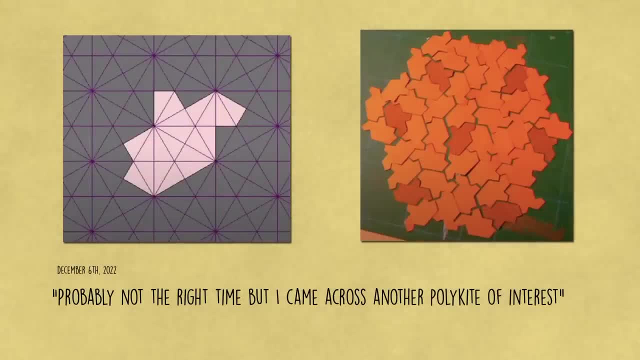 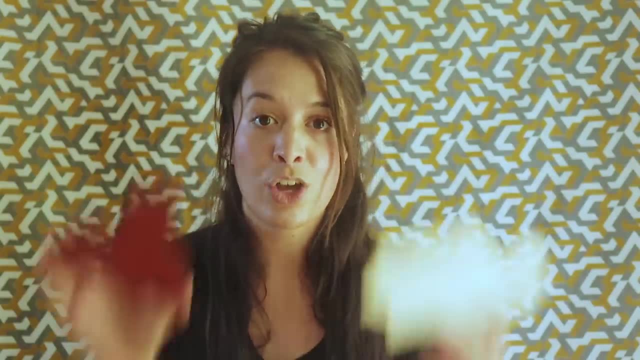 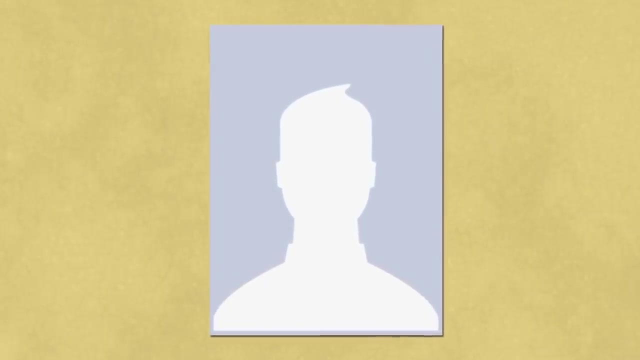 Probably not the right time, but I came across another polychite of interest. It's called the Turtle, for obvious reasons. After a 50-year dry spell, suddenly two different Einstein tiles. As if that wasn't enough, it was here that Joseph had an incredible insight. 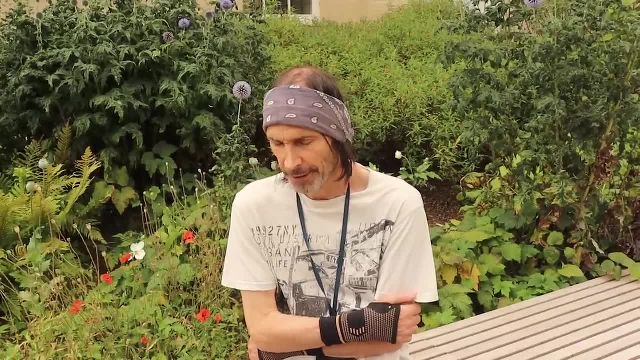 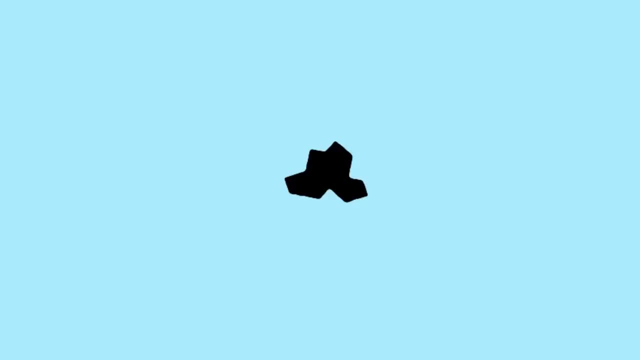 Joseph. I mean, he's like- um, I don't know what else to say- He's like, he's like an artificial intelligence. Yeah, The hat and the turtle were related. By adjusting the lengths of the sides, you can morph the hat into the turtle. 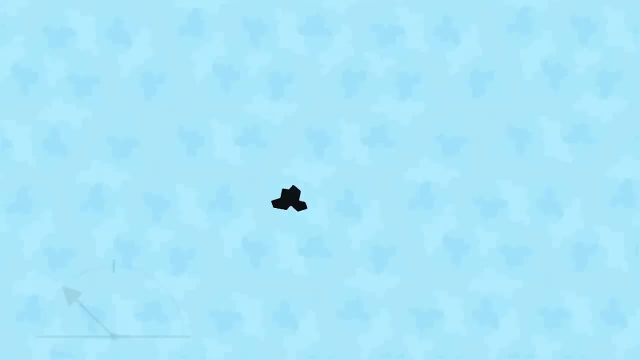 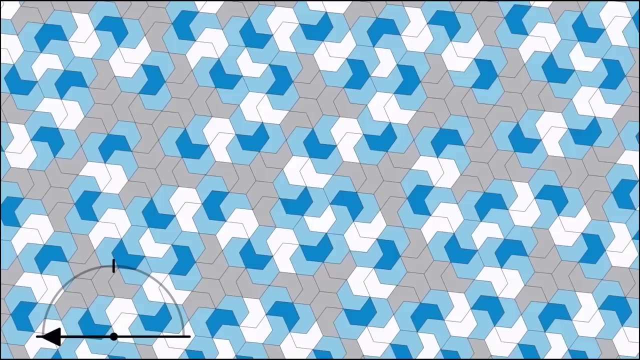 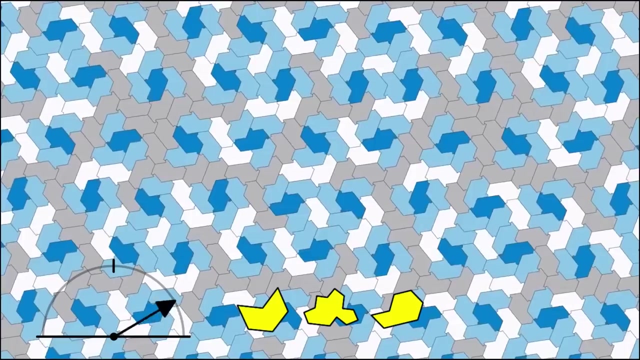 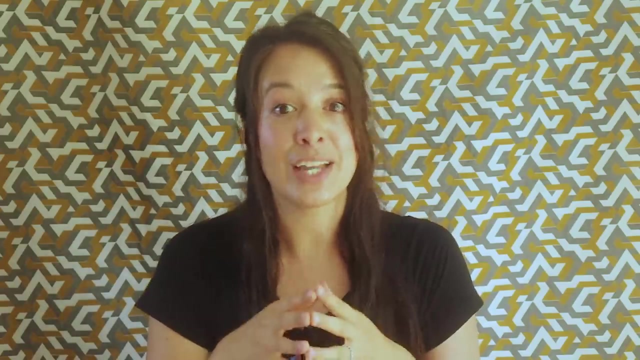 and the turtle into the hat. Not only that, but this gives an infinite continuum of aperiodic monotiles. Except for the shapes at the extremes, every single shape in this morphing continuum tiles the plane aperiodically. For 50 years we didn't have a single aperiodic monotile, and now we have infinitely many. 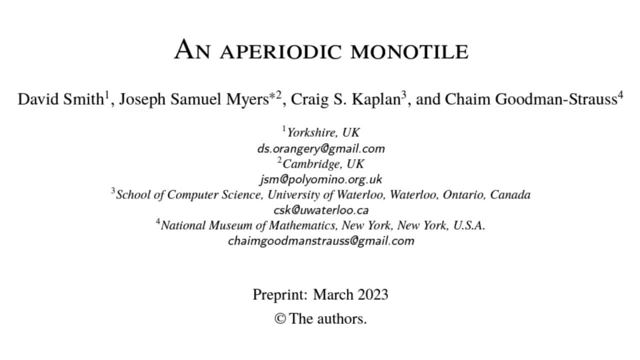 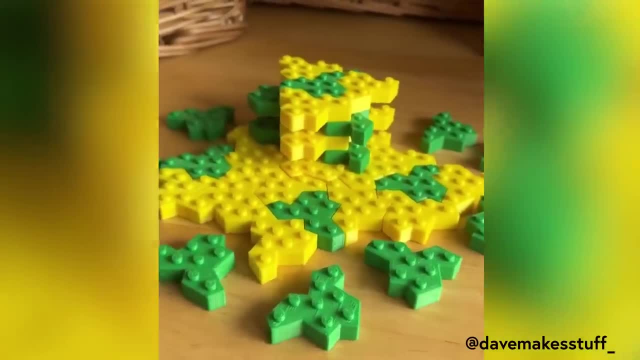 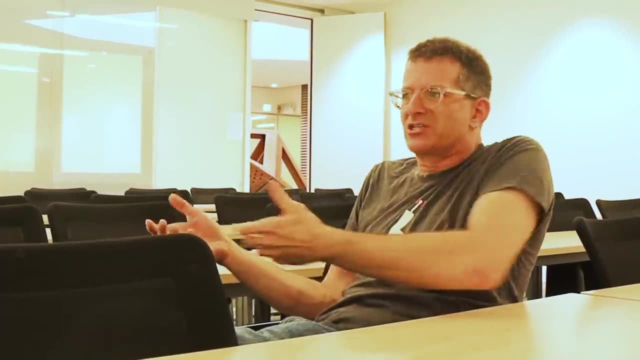 The result was published in March 2023. So yeah, Just five months after Dave discovered the hat, It took the math world by storm. People could not stop celebrating. We finally have the well, the happy ending to this long story, this quest. 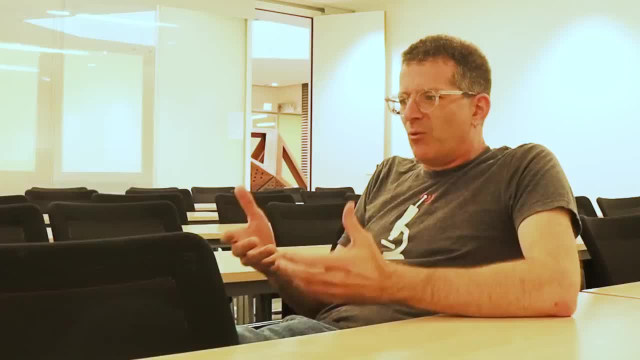 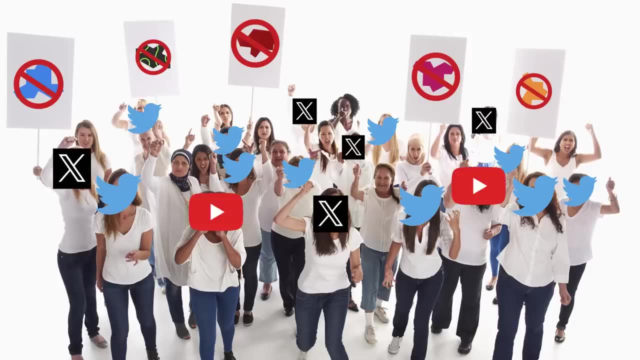 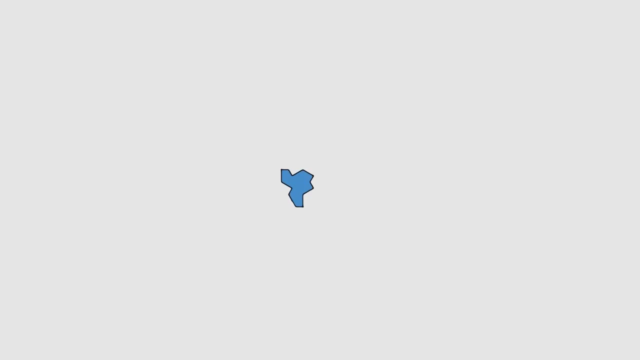 Except it wasn't the end of the story. Some people weren't happy with these tiles, And by some people I mean Twitter And some of you guys. I posted a YouTube short about the Einstein tile earlier this year, and the reoccurring complaint was that it doesn't count as a single tile. 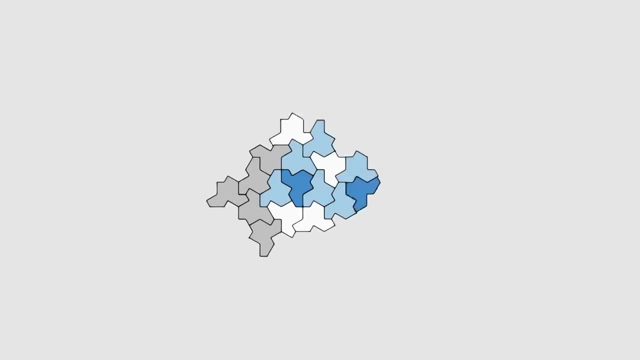 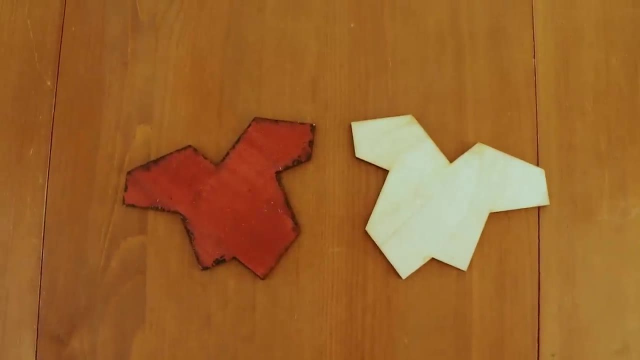 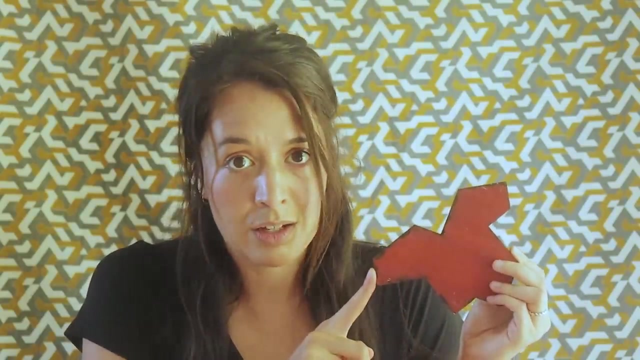 because it uses its reflection. I do understand this complaint. If you wanted to tile your bathroom floor with it, you'd need two different tiles made, So people were arguing that this wasn't really the Einstein tile. How did I personally feel about it? 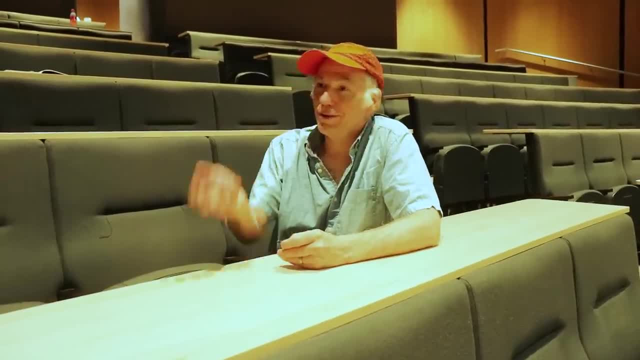 Well, I guess on some level it wasn't the Einstein tile. Well, I guess on some level it wasn't the Einstein tile. Well, I guess on some level it wasn't the Einstein tile. I guess on some level it's like: well, come up with your own tile, then, buddies. 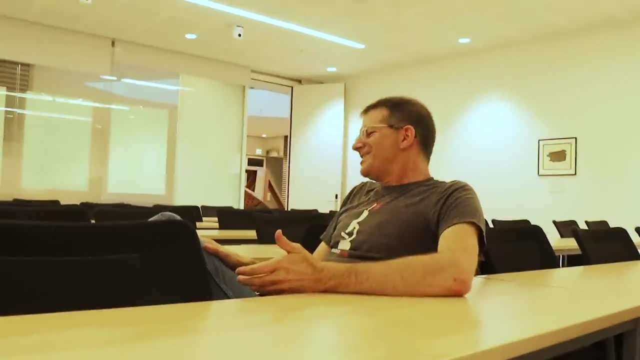 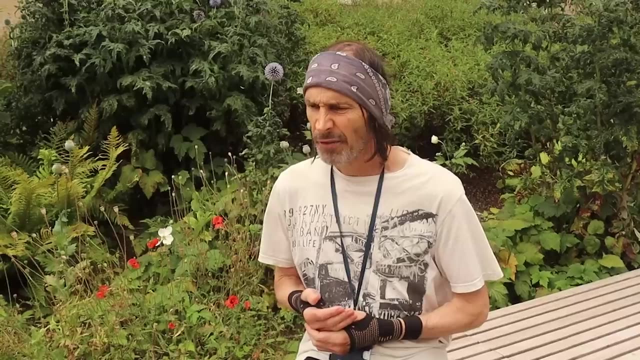 That I mean haters gonna hate. I don't know right, I was a bit cheesed off about it really, Because there was a lot of people that were just basically moaning. But whether or not you think a shape in its reflection is one or two shapes, 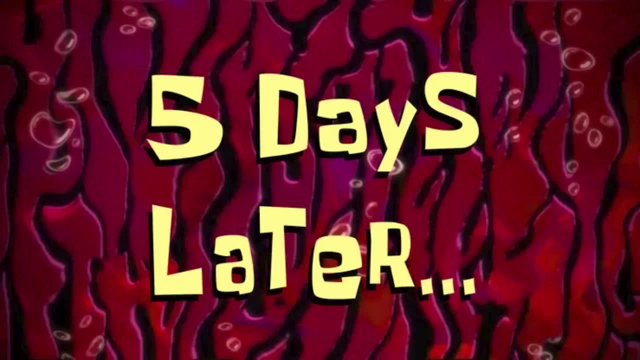 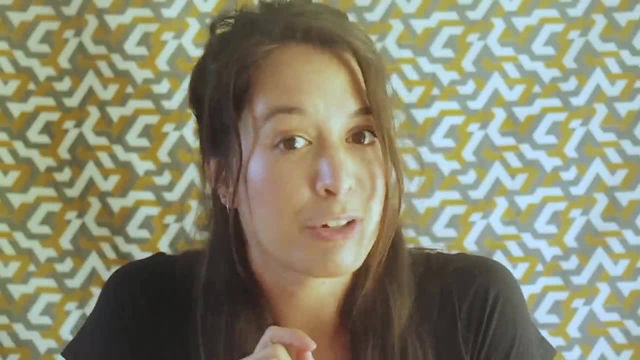 doesn't matter anymore, Because just five days after the paper was published, Dave found another aperiodic monotile, And this one does not count, It does not need its mirror reflection. For those who thought the hat was two tiles, this is one. 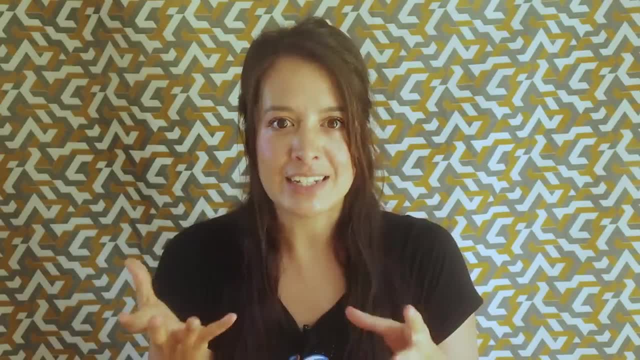 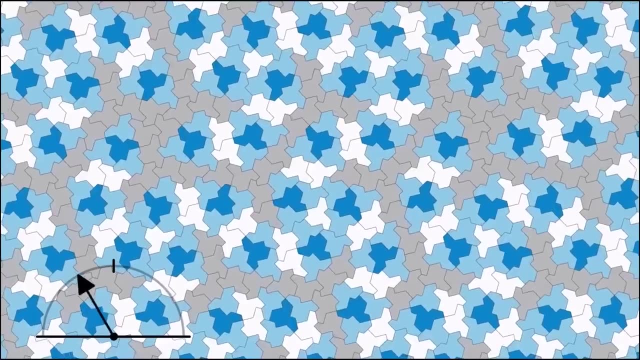 They've got nothing to moan about on it. It was hiding in plain sight, yet nobody recognised it, Except Dave. It was in front of everyone's eyes. You know how I said that all these shapes tile aperiodically, except the ones at the extremes. 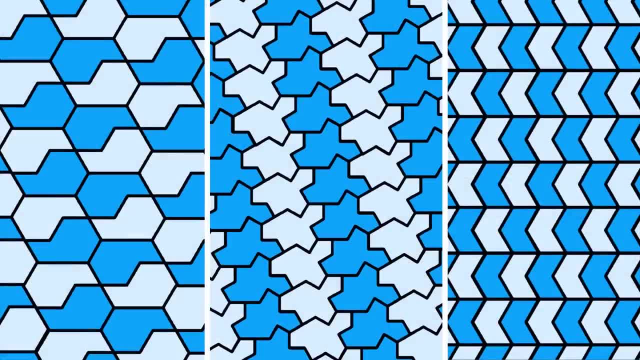 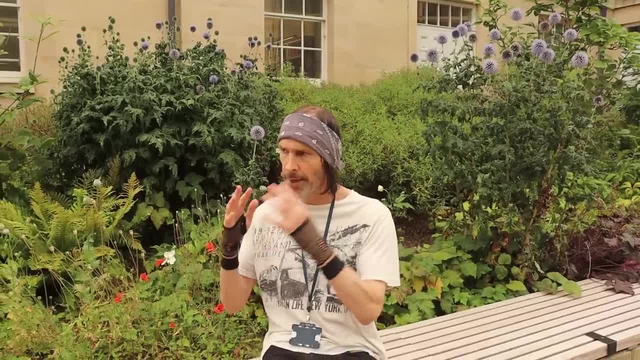 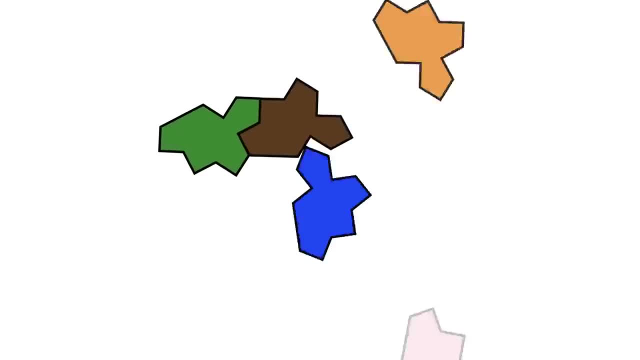 They tile periodically, Which is not that exciting. Yet somehow this particular shape Caught Dave's eye. I kind of put it together in my head, You know, assembled it in my head, And I think, hang on a minute, this has more freedom than the hat. 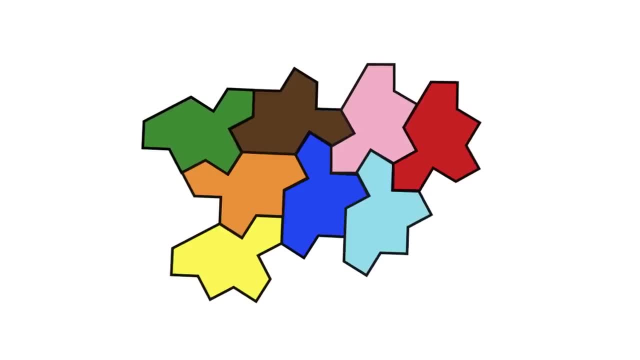 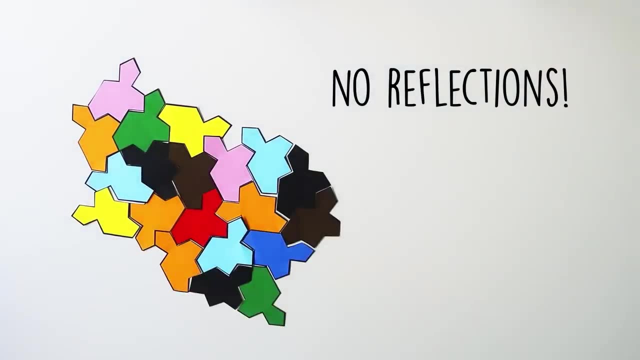 Which is understandable because it's periodic. And so I thought, well, maybe I should just cut them out and play with just a front or a back, Don't flip them. And I kind of did that And an aperiodic pattern emerged. 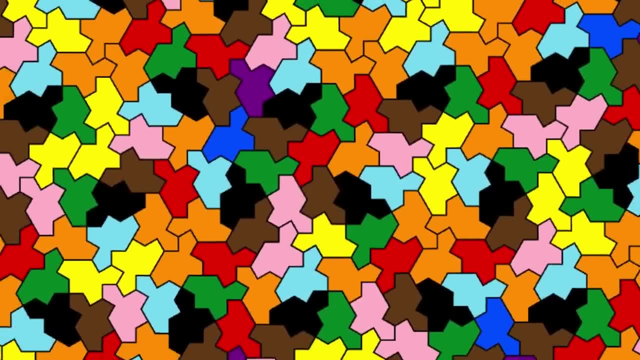 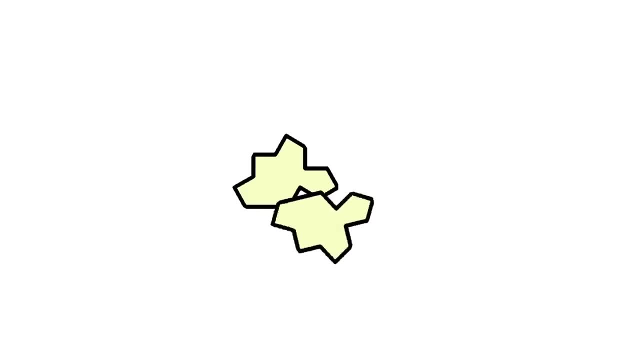 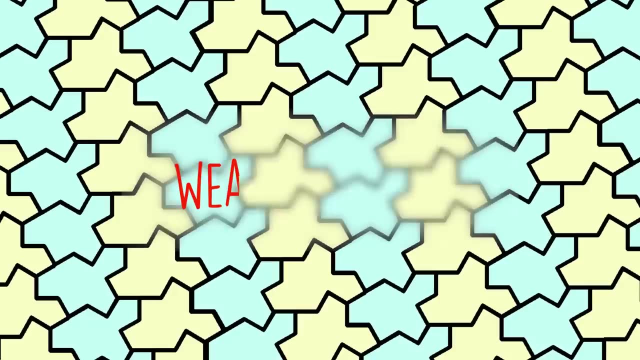 So here we have a single tile That doesn't use its mirror reflection. that tiles the plane aperiodically. However, when you include its mirror reflection, it does tile periodically. So the researchers said that this shape was weakly aperiodic. 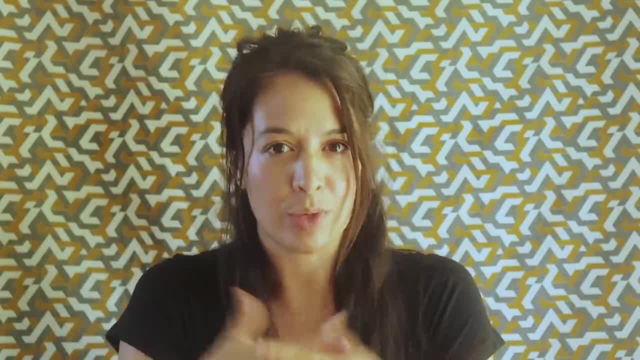 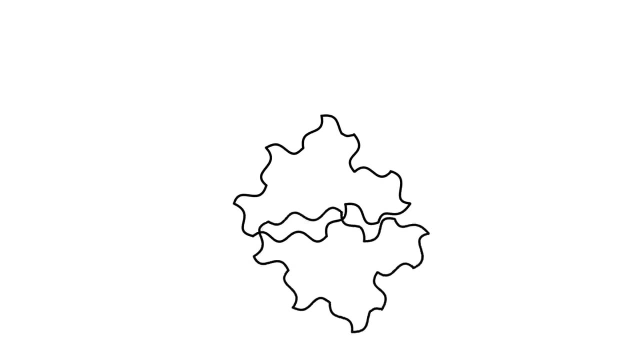 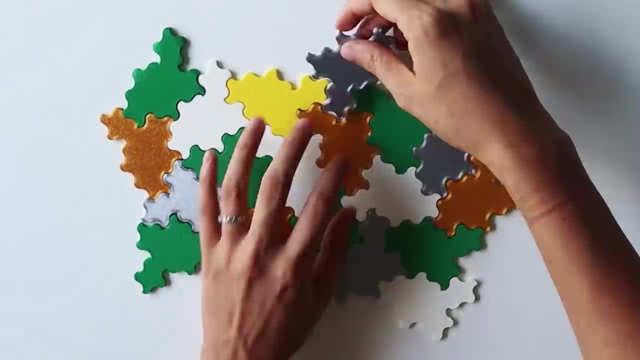 Ideally, they wanted a shape that does not tile periodically with its mirror image, But they solved this problem by wiggling its sides. Now it no longer fits with its mirror reflection And still fits, But it still tiles aperiodically. If you wanted to get your bathroom floor tiled, you'd only need to get one shape made. 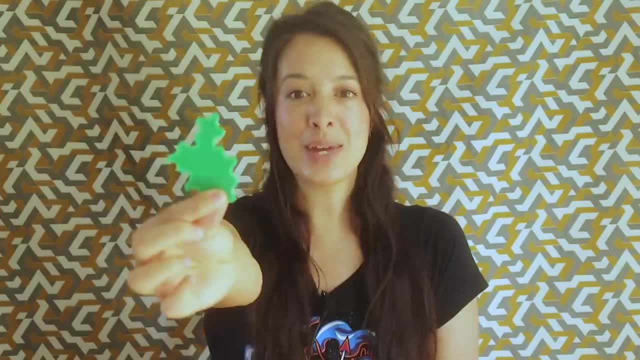 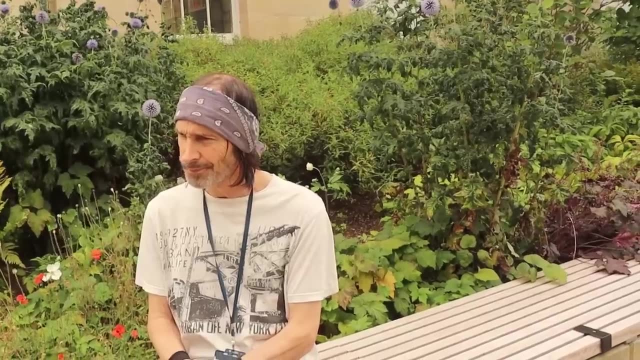 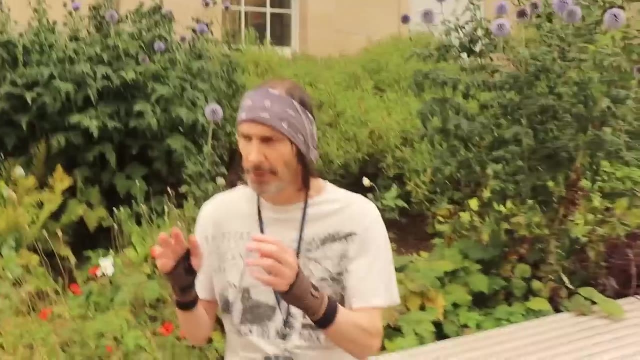 So here we have an undisputable Einstein tile. It's called the Spectre. Why did you call it the Spectre? Ah, yeah, Well, I think because it was in between my brother's, my oldest brother's, death. The Spectre is like a spirit or a presence. 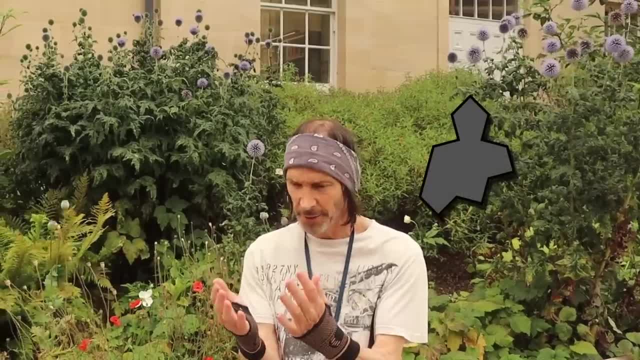 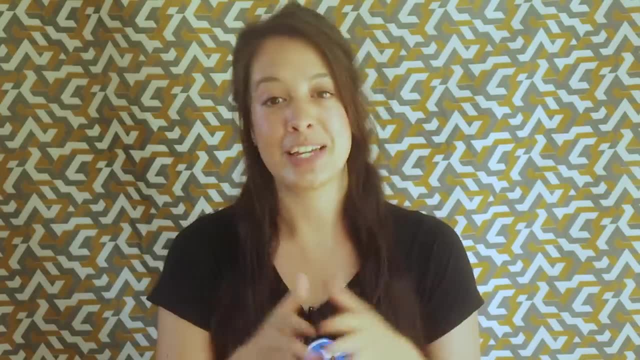 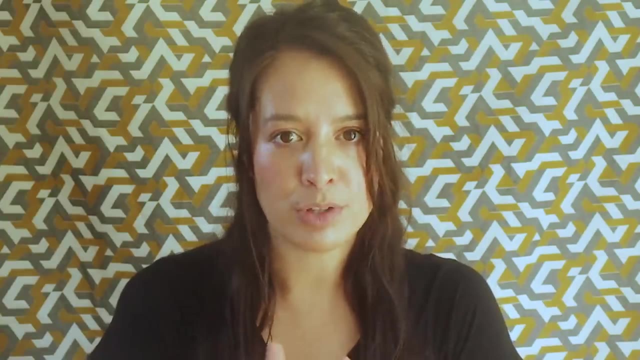 And I felt it. I could see it. This thing was looking over me. It was just this figure Looking over me. This is a groundbreaking mathematical discovery and I would be happy to leave the video here, But I knew a lot of you wouldn't be happy unless I talked about possible practical applications. 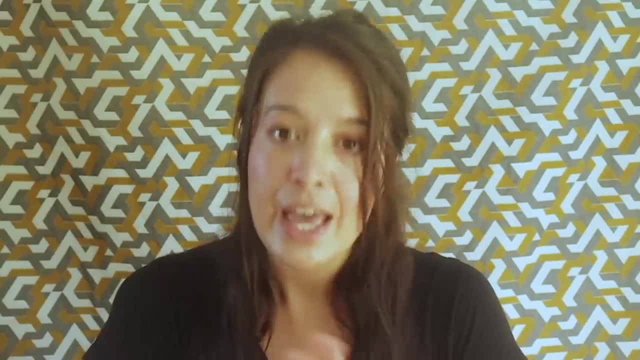 It turns out that, apart from making a cool bathroom floor, aperiodic patterns are being used to make new materials. Physicists will be quite excited about a few properties of it. Materials with periodic lattices have been used to make new materials. 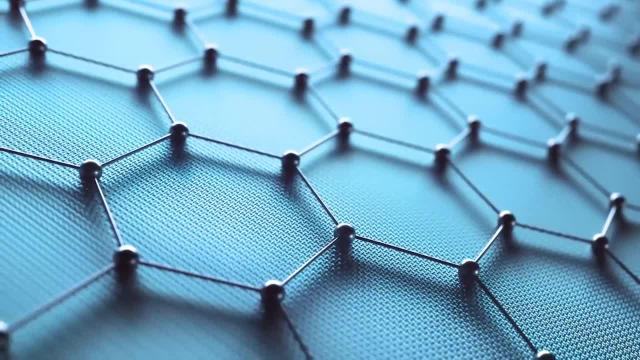 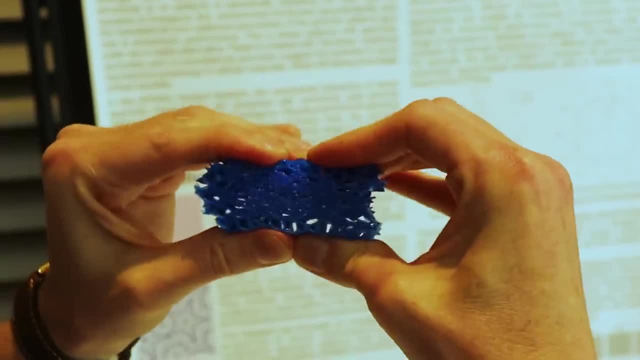 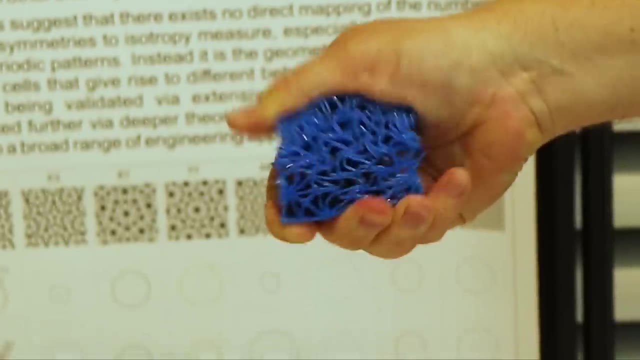 Materials with periodic lattices have been used and studied extensively in material science and engineering, And now scientists are experimenting with aperiodic lattices. They've found that they behave in different and surprising ways. We're only a few months in, but already they're finding that they may be more elastic and less prone to failure than their periodic ancestors. 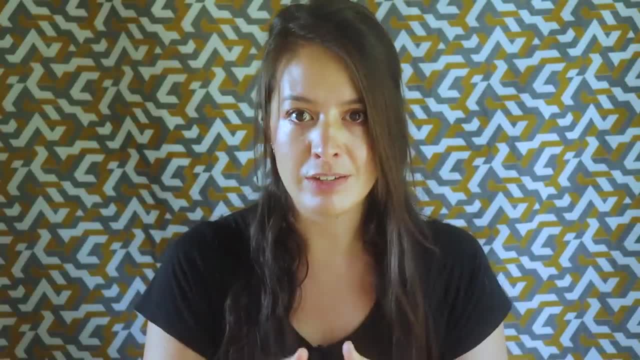 We're still discovering applications for the Penrose tiles, and they were found over 50 years ago. Given time, who knows what other cool inventions the Einstein tile could lead to? Given time, who knows what other cool inventions the Einstein tile could lead to? 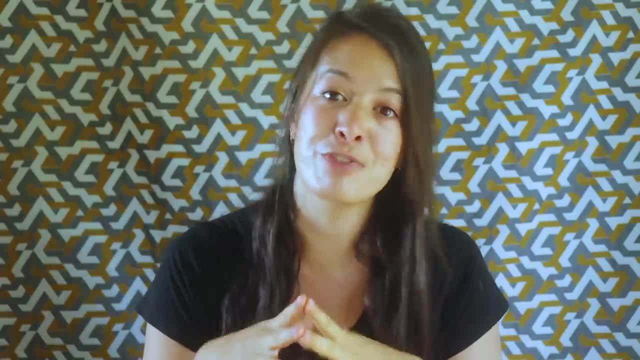 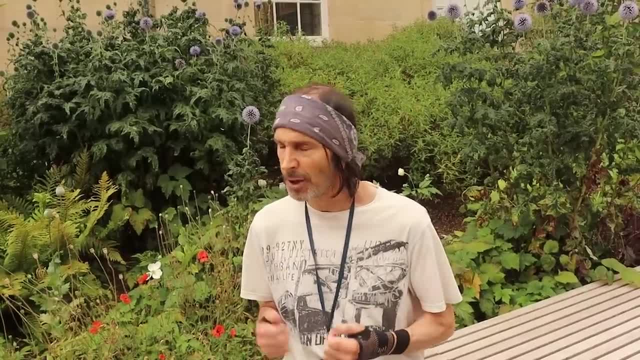 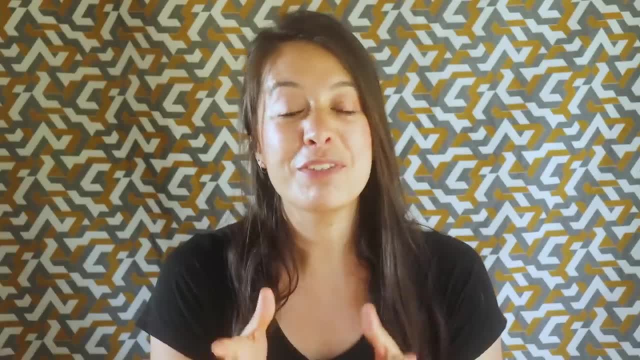 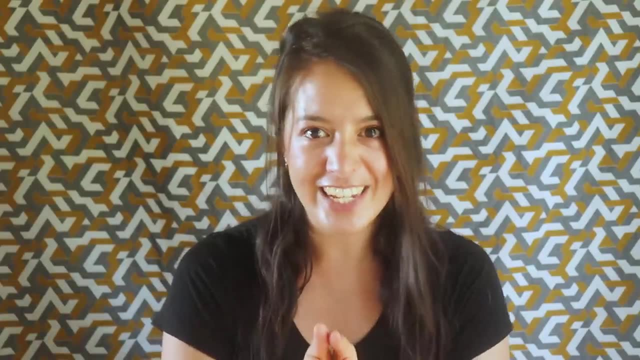 In the meantime, if you did want to get your bathroom floor tiled, here's what Dave has to say about that one. dave is one of the most inspiring parts of this story. without any formal training in mathematics, he contributed to a groundbreaking discovery. it just goes to show that anyone can. 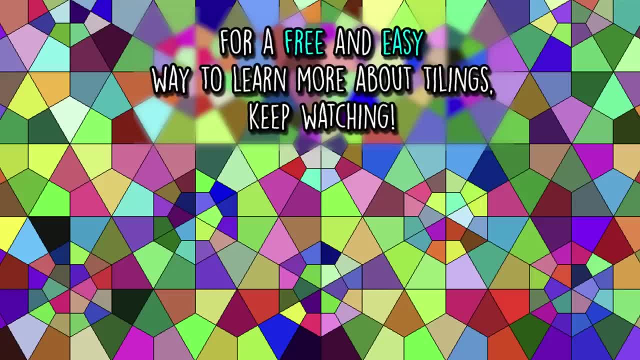 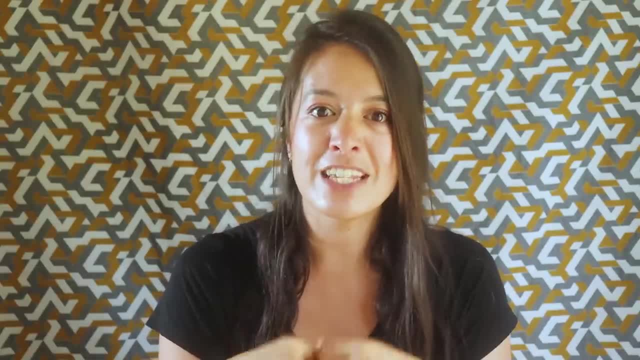 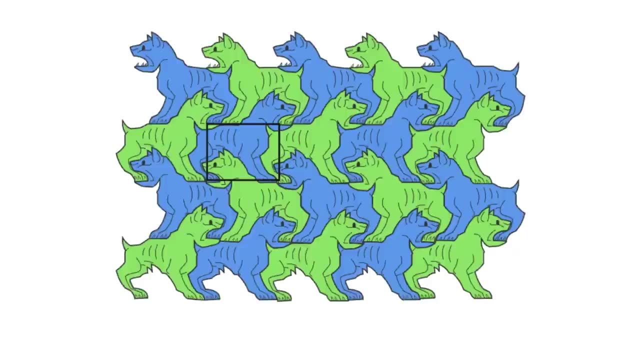 dive into and even influence the world of math. because they're so visual, tilings offer an accessible gateway into math. i've become a bit obsessed and i'm loving this beautiful geometry course on brilliant. if you've been captivated too, i highly recommend it. in this course you'll